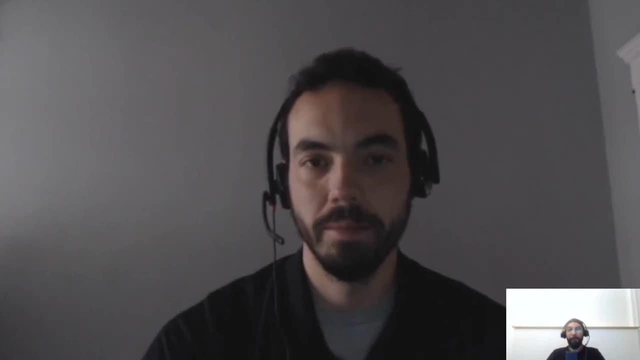 Yeah, So also you have a really diverse skill set and you have been associated with robotics for such a long time, So you can probably give a good view on what are the skills one should have for robotics. Of course, you know, the tools is a different thing and skills is a different thing. 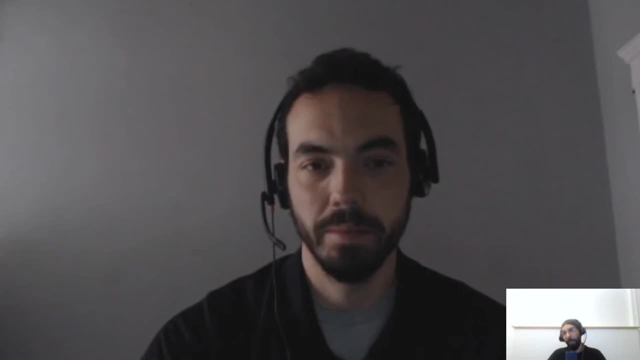 So what are the skills that you know one must have to have to be a good roboticist? Yeah, So two of them I think we already touched on. One was just the systems thinking. You need to have a baseline level of systems thinking because, in robotics especially so, you don't have the luxury of saying, oh, that's not my area of expertise, Therefore, let me ignore it. 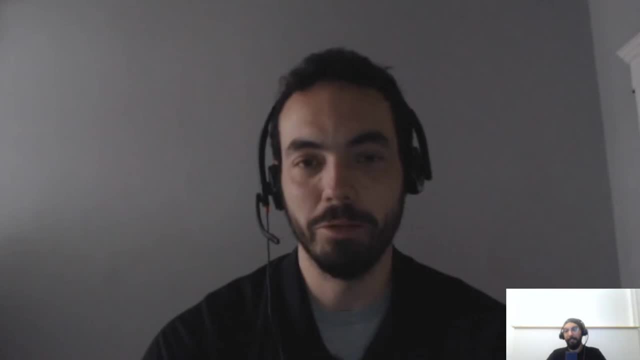 You need to understand a lot of different things, because robots are complicated systems. It is what it is. Another skill that we already talked about was the whole like: don't just learn tools Or languages. for the sake of it, Don't take a tools-focused approach, Take a problem-focused approach. I'll leave it at that. But you know a lot of newcomers will ask things like: oh, what's the best programming language to learn? You know, is it C++, Is it MATLAB, Is it Python? It really depends on what you want to do. I mean, just I would say: what are you trying to solve, right? 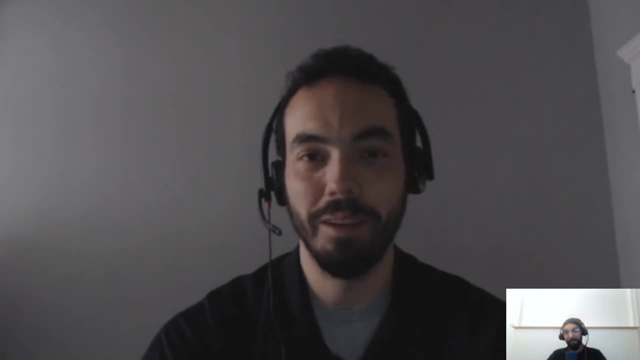 If you're trying to write a piece of software that goes in a microcontroller, then you're probably going to want to use C, you know, and so on, Although one software tool that I would recommend everyone learn in robotics is ROS. Actually, my current boss at Boss Dynamics said this really well and I want to share it with people- is that for most robotics companies out there, if you're working on software, even if they're not using ROS, there is going to be something like it. 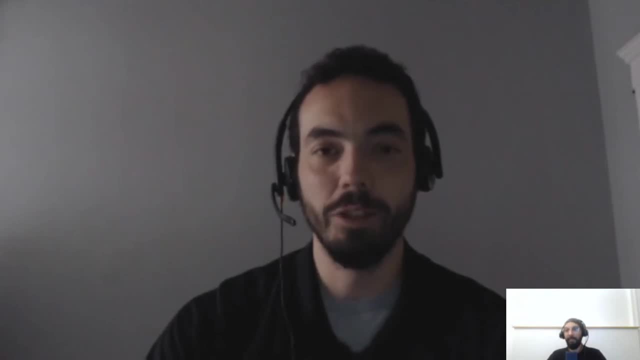 So it's really good to just have that knowledge of, like you know, splitting up your software into different distributed nodes and serializing messages or serializing data in the form of messages and so on, A framework of any Sort, basically. 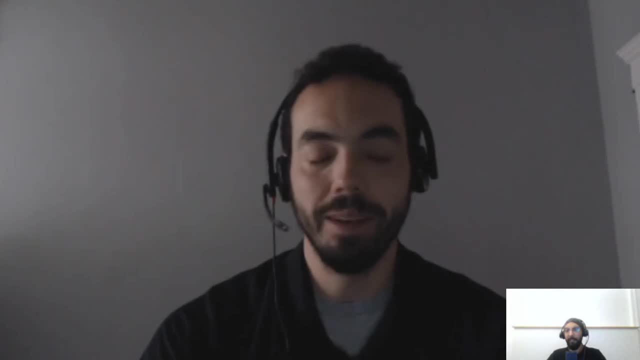 Yeah, yeah, So there's that. I mean, you know my advice is focused on the software side, because that's what I've been doing most of my time. The third one is- and I got this from a book about the Google software engineering process, which is. I forget who writes it, but it's called The Flamingo Book.